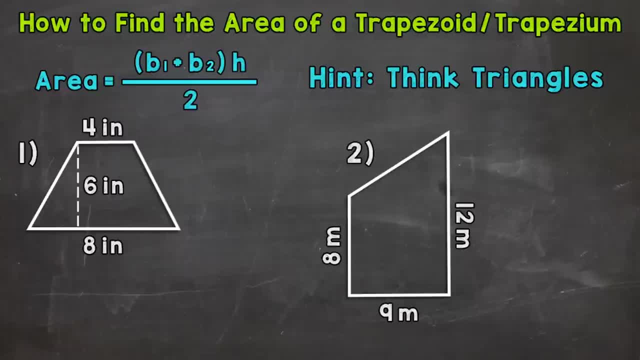 Now remember, a trapezoid is a quadrilateral with one pair of parallel sides, And the formula we use to find the area is the length of base 1 plus the length of base 2 times the height divided by 2.. Hint, think triangles. I'll show you exactly what I mean by that. 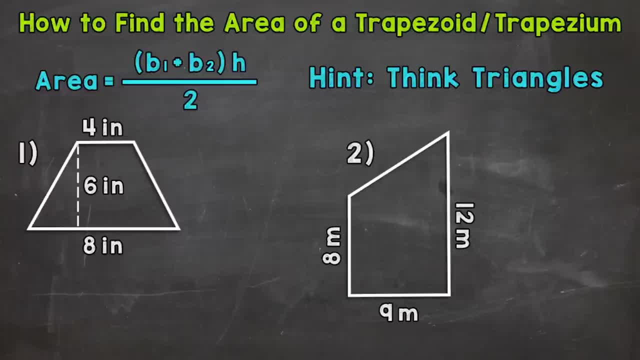 as we go through our examples Now, when we're talking trapezoids, the bases are going to be the parallel sides. It doesn't matter if it's the top, bottom side or other side. It matters which sides are parallel. 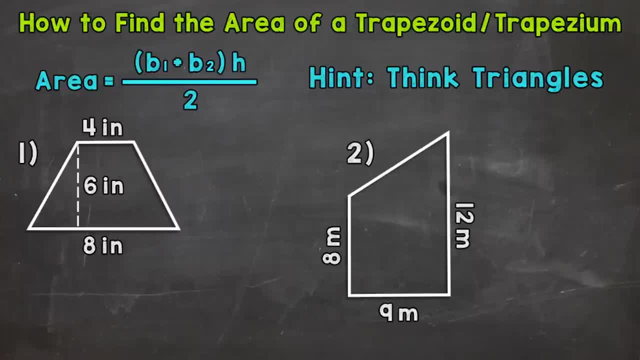 Those are your bases. The other sides, which are not parallel, those are called the legs. So let's jump into number one, where we have a trapezoid with the bases at the top and bottom and then these sides that are not parallel, these are the legs. We will not need the measurements. 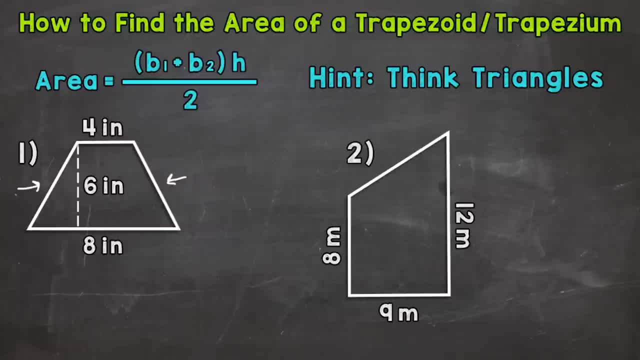 of those legs to calculate the area. So we're going to write out our formula and plug in the information we need. So area equals, Well, base 1 plus base 2, times the height of the trapezoid divided by 2.. So let's plug in. 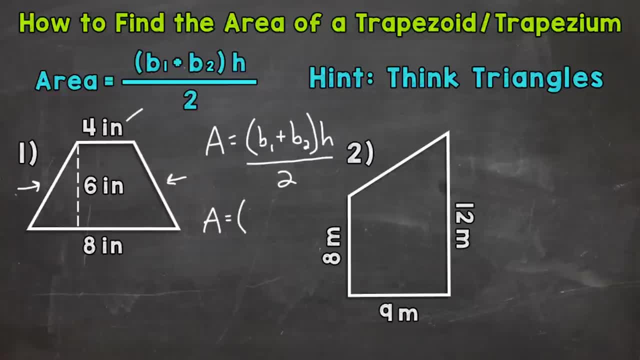 Base 1, we're going to use 4 inches Plus base 2, we're going to use 8 inches. Remember, the bases are the parallel sides. times the height, which is 6 inches, Divide it by 2.. So we have 4 plus 8, which is 12, times 6 is 72. So we have 72 over 2, or 72 divided by 2.. 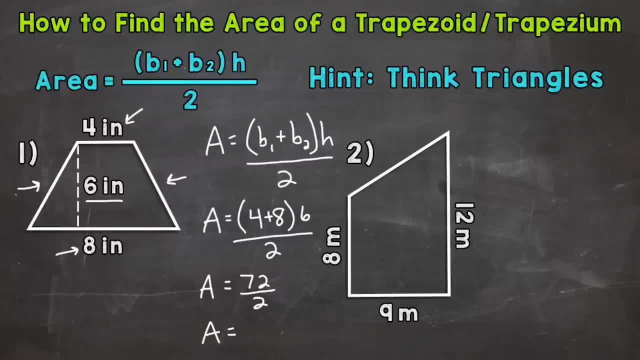 Our final area is going to be: well, 72 divided by 2 is 36, and this is square inches because we're talking area. So 36 square inches for the area for number 1.. Now you may have noticed that the formula we use to find the area of a trapezoid is similar to the formula we use to find the area of a triangle. 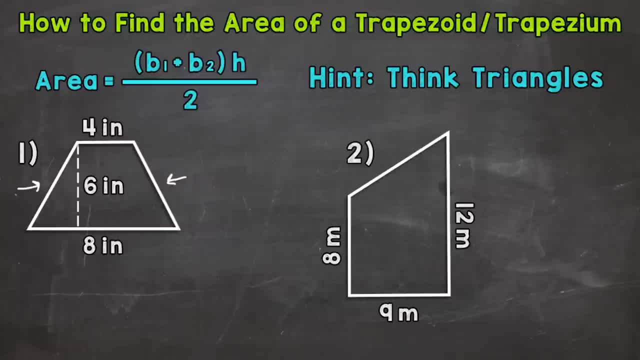 of those legs to calculate the area. So we're going to write out our formula and plug in the information we need. So area equals, Well, base 1 plus base 2, times the height of the trapezoid divided by 2.. So let's plug in. 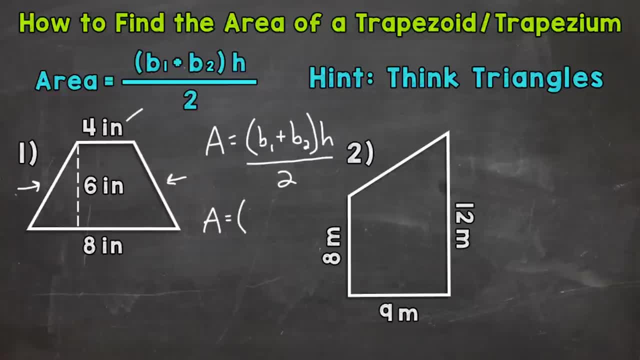 Base 1, we're going to use 4 inches Plus base 2, we're going to use 8 inches. Remember, the bases are the parallel sides. times the height, which is 6 inches, Divide it by 2.. So we have 4 plus 8, which is 12, times 6 is 72. So we have 72 over 2, or 72 divided by 2.. 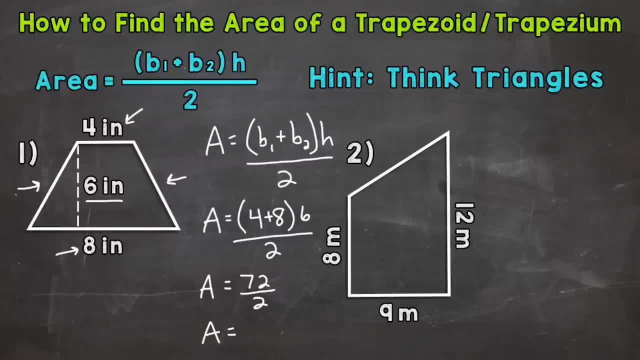 Our final area is going to be: well, 72 divided by 2 is 36, and this is square inches because we're talking area. So 36 square inches for the area for number 1.. Now you may have noticed that the formula we use to find the area of a trapezoid is similar to the formula we use to find the area of a triangle. 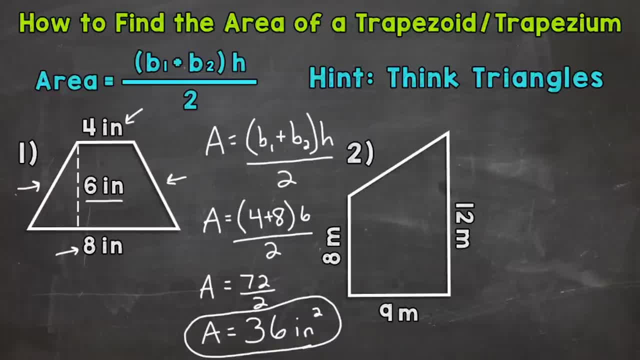 The area of a triangle is base times height divided by 2, or 1 half times the base times the height. Multiplying by a half is the same as dividing by 2, so if you see those different formulas, they mean the same thing. 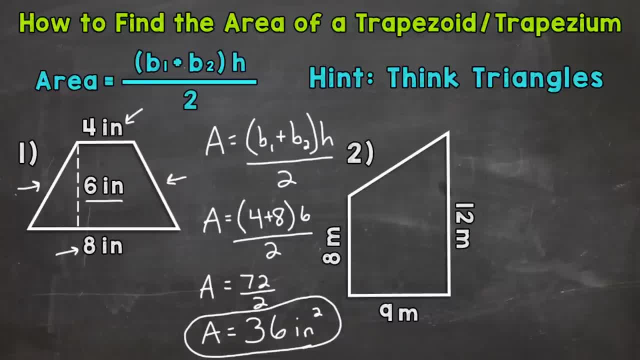 But for this we have base 1 plus base 2 times height divided by 2.. I'll show you why. So trapezoids can be split into two triangles. For example, number 1, if I go from one corner to the other. 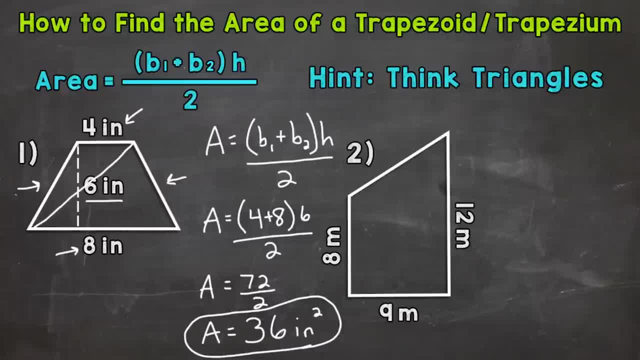 so top right to bottom left, I get two triangles. I'd get two triangles if I went from the top left to the bottom right as well, so it doesn't really matter which of those you use. It will split or divide that trapezoid into two triangles. 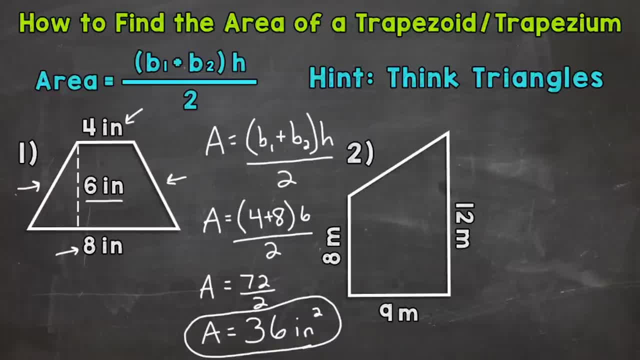 The area of a triangle is base times height divided by 2, or 1 half times the base times the height. Multiplying by a half is the same as dividing by 2, so if you see those different formulas, they mean the same thing. 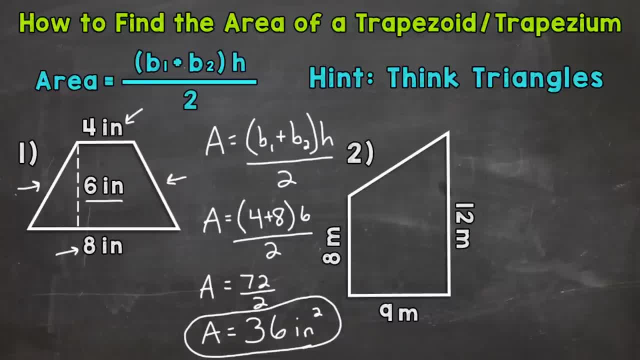 But for this we have base 1 plus base 2 times height divided by 2.. I'll show you why. So trapezoids can be split into two triangles. For example, number 1, if I go from one corner to the other. 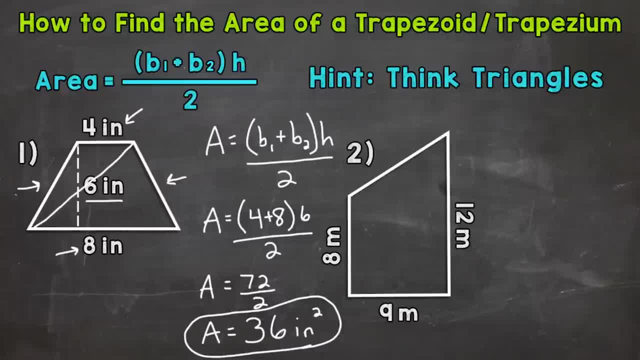 so top right to bottom left, I get two triangles. I'd get two triangles if I went from the top left to the bottom right as well, so it doesn't really matter which of those you use. It will split or divide that trapezoid into two triangles. 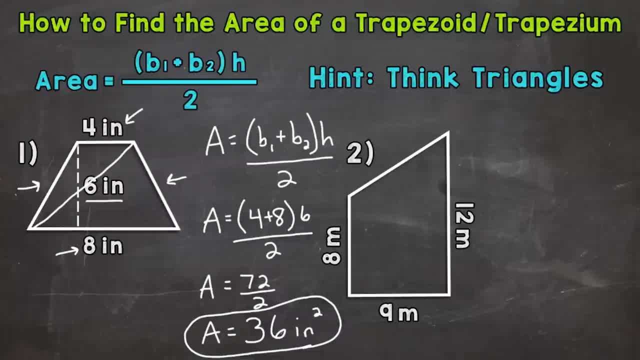 Now the triangles' bases will be the same as the trapezoids. they will correspond and the height of the triangles will be the same as the trapezoid as well. So what we could do, we could find the area of those two triangles and add them together to get the area of the trapezoid. 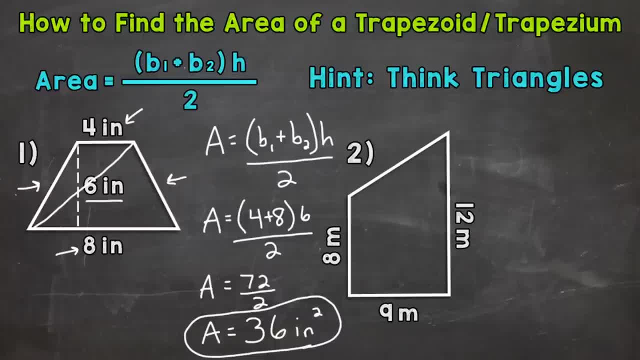 But we can combine that process in the one formula, which is what we just did when we did base1 plus base 2 times the height divided by 2.. Let's move on to number 2, and we'll start by writing out our formula, So area. 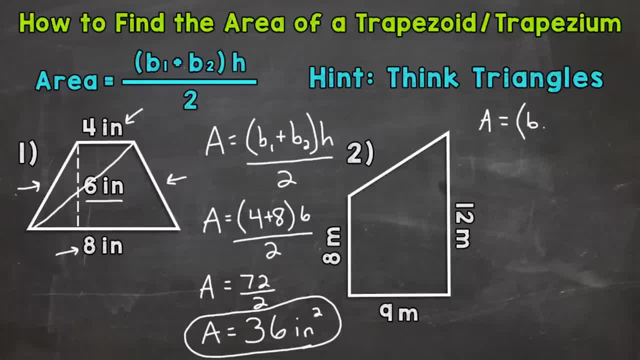 equals base 1 plus base 2 times the height divided by 2.. So let's plug in. So base 1,. well, we need to find the two parallel sides, and the two parallel sides are the 8 meters and the 12 meters. It doesn't really matter which one you use for base 1 or base 2, because adding 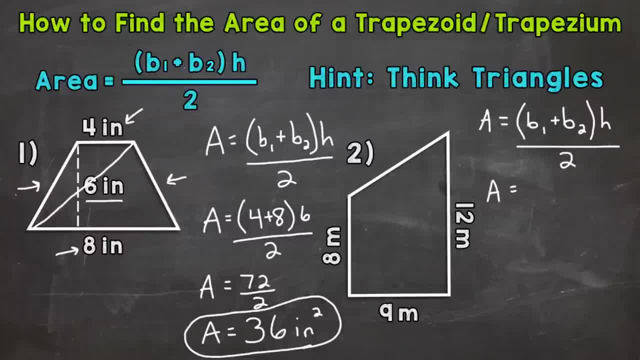 them together- 12 plus 8 or 8 plus 12, is going to give you the same thing. I'm going to use 8 for base 1 and 12 for base 2.. So 8 plus 12 times the height of 9 meters. In this problem we'll. 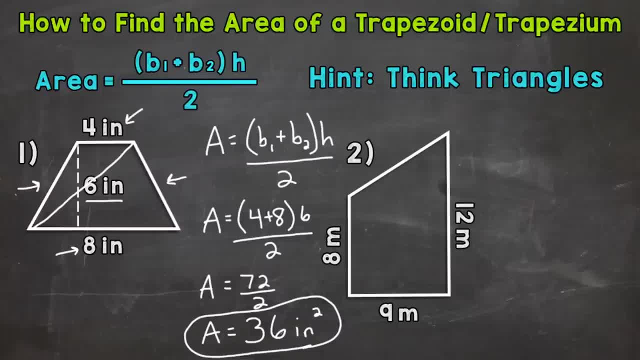 Now the triangles bases will be the same as the trapezoids. they will correspond and the height of the triangles will be the same as the trapezoid as well. So what we could do: we could find the area of those two triangles and add them together to get the area of the trapezoid. 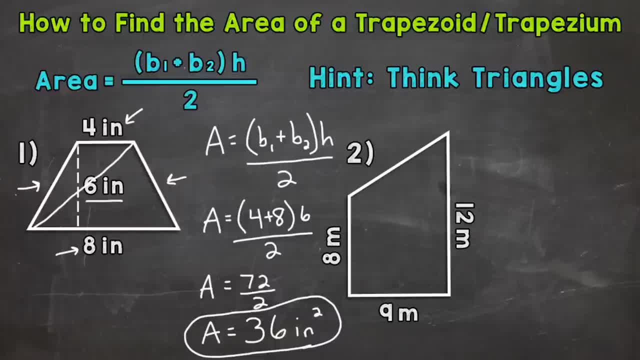 But we can combine that process in the one formula, which is what we just did when we did base 1 plus base 2 times the height divided by 2.. Let's move on to number 2, and we'll start by writing out our formula, So area. 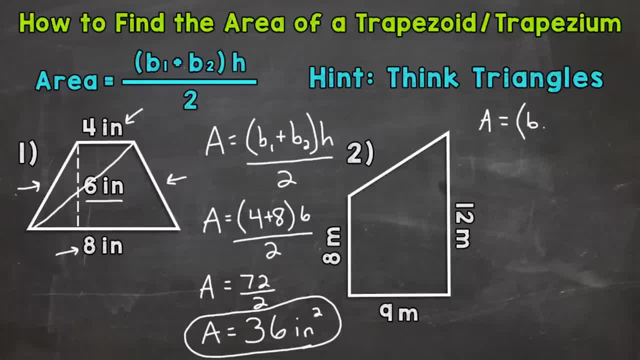 equals base 1 plus base 2 times the height divided by 2.. So let's plug in. So base 1,. well, we need to find the two parallel sides, and the two parallel sides are the 8 meters and the 12 meters. It doesn't really matter which one you use for base 1 or base 2, because adding 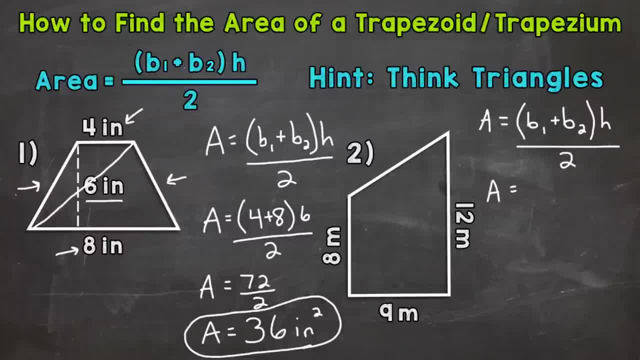 them together- 12 plus 8 or 8 plus 12, is going to give you the same thing. I'm going to use 8 for base 1 and 12 for base 2.. So 8 plus 12 times the height of 9 meters. In this problem we'll. 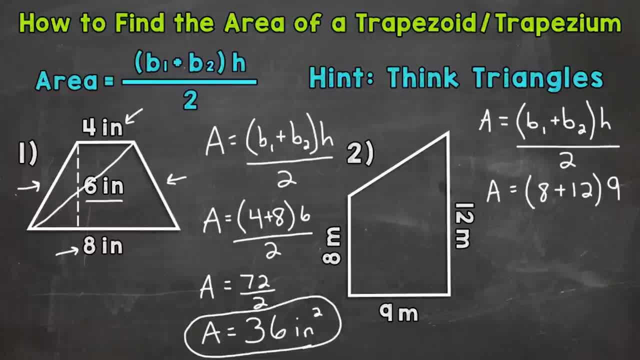 use the measurement of one of the legs In number 1, we didn't need any of the measurements for the legs, but number 2, one of those legs gave us the height, So we used it and we divide that by 2.. So we know that 8 plus 12 is 20 times 9 is 180, and we divide that. 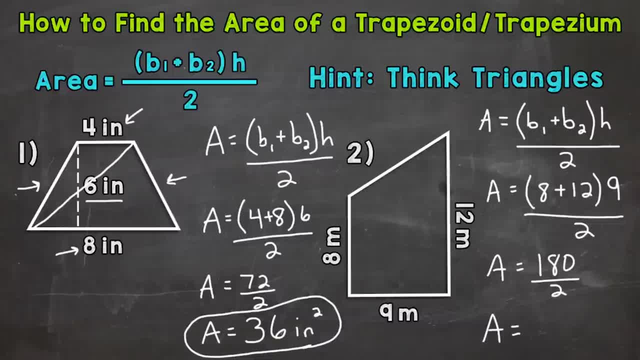 by 2 to get our final area. So 180 divided by 2, or half of 180, is going to be 90. And that is square meters. So that's our area for number 2.. And let's take a look what happens. 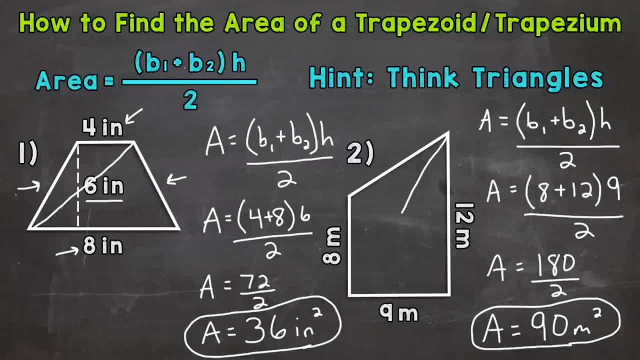 when we split this into two triangles. just to get another visual, I'm going to go top right to bottom left again and you can see that that trapezoid was divided into two triangles. So that formula helps us combine the areas of both of those triangles to get the final area. Now again,